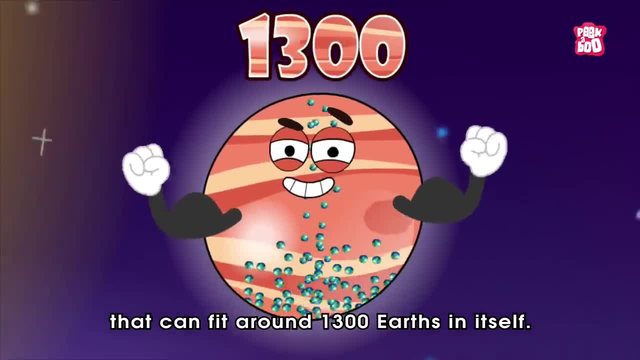 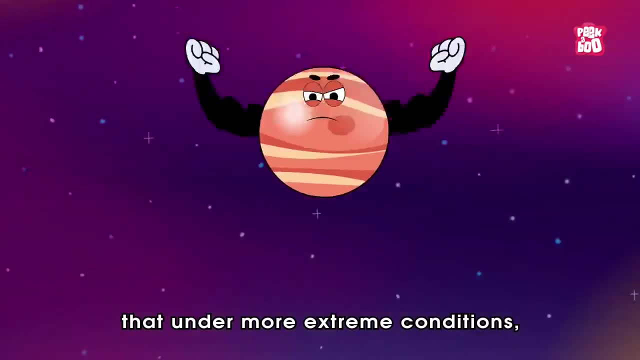 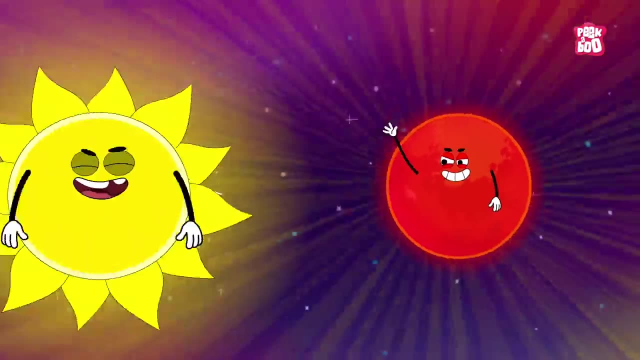 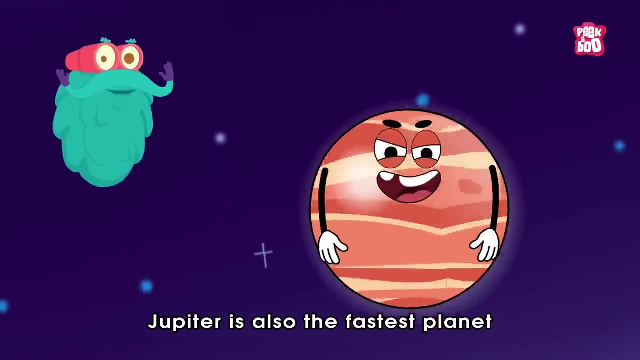 that can fit around 1,300 Earths in itself. Due to this massive size, scientists assume that under more extreme conditions, Jupiter could have evolved into a dove, A double star companion to our Sun. And despite being so huge, Jupiter is also the fastest planet in the solar system. 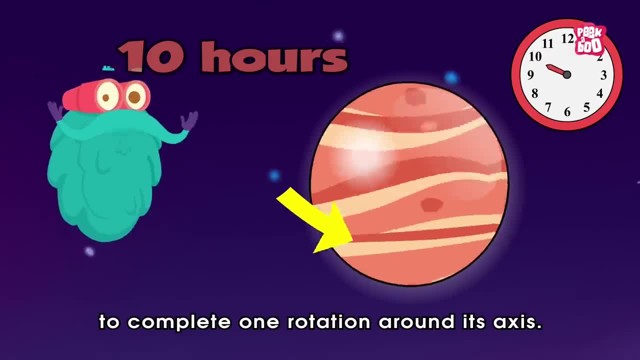 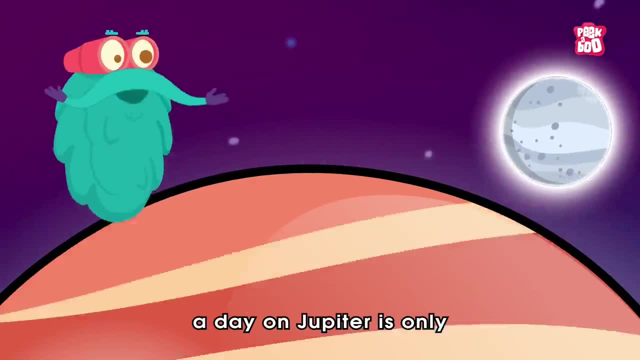 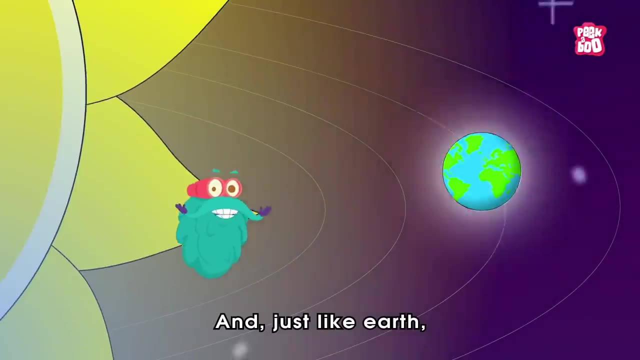 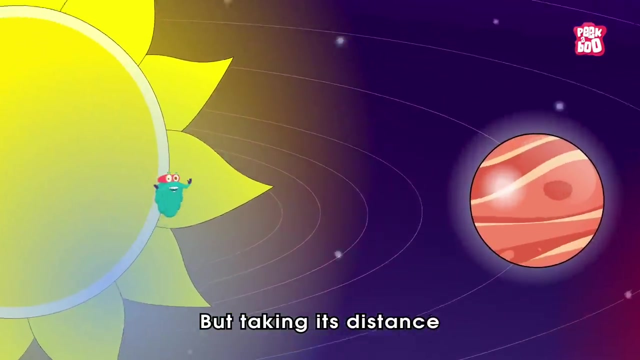 as it takes only 10 hours to complete one rotation around its axis, Meaning a day on Jupiter is only 10 hours long, versus 24 hours on Earth, And, just like Earth, Jupiter rotates around the Sun in an elliptical orbit, But taking its distance from the Sun into account. 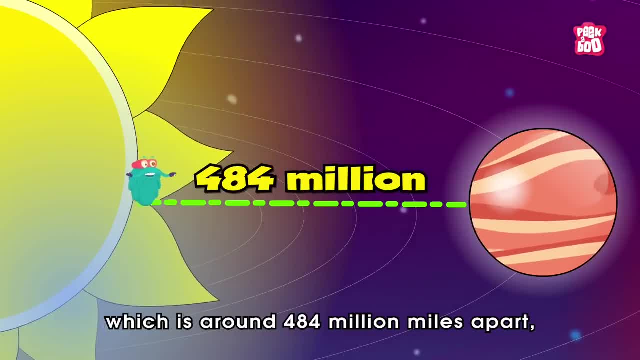 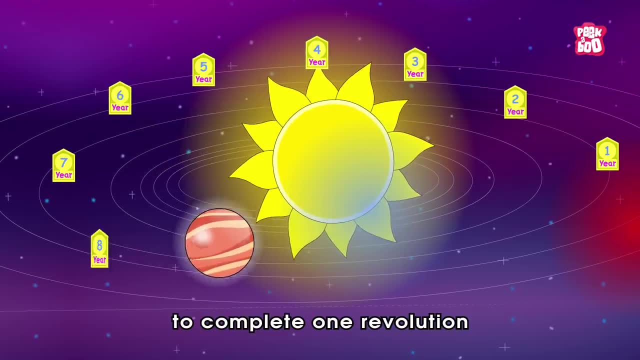 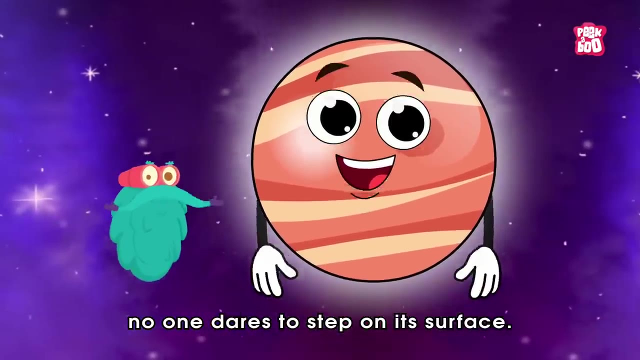 which is around 484 million miles apart. it takes a whopping 12 Earth years to complete one revolution around the Sun And for all these reasons, no one dares to step on its surface. Why To know about it? please check out our video. 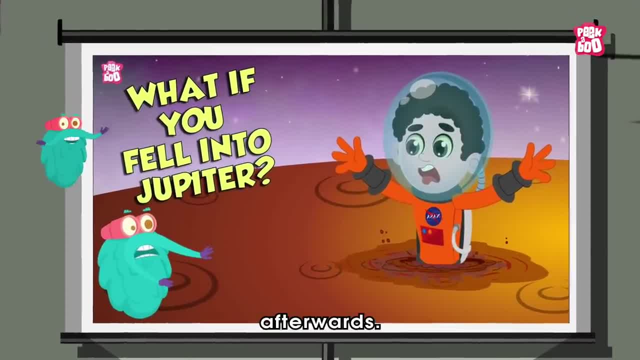 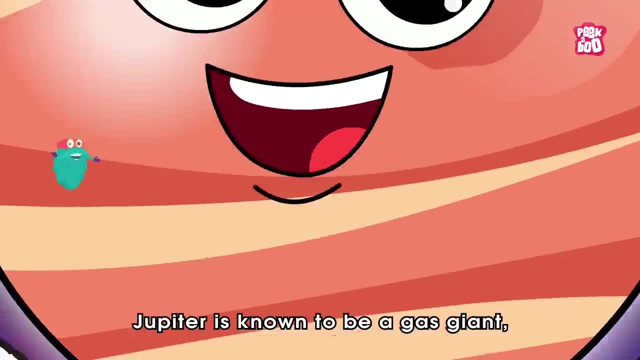 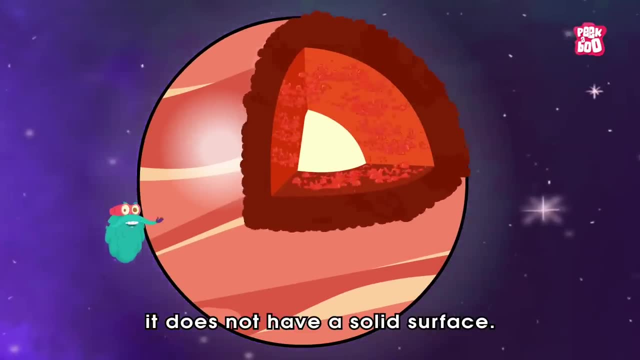 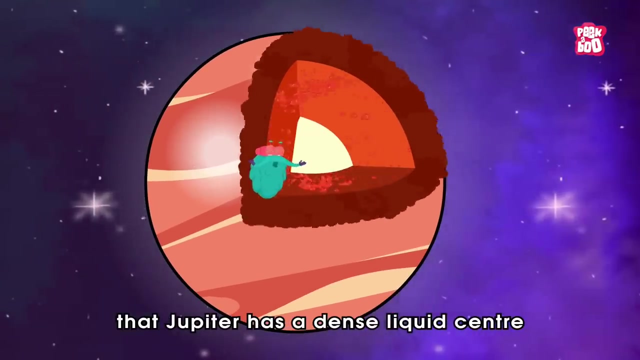 What if you fell into Jupiter afterwards? But to give you an idea, it is because Jupiter is known to be a gas giant And, unlike the Earth and the other terrestrial planets, it does not have a solid surface. Also, some scientists suggest that Jupiter has a dense liquid center. 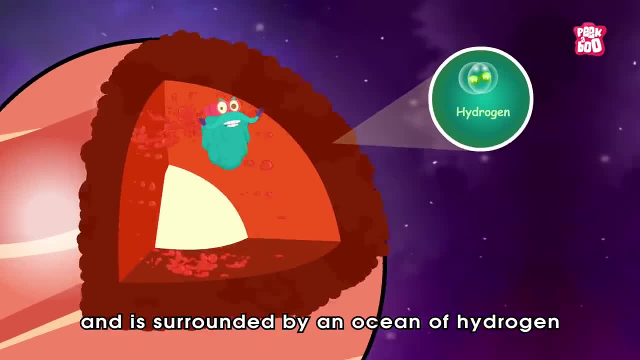 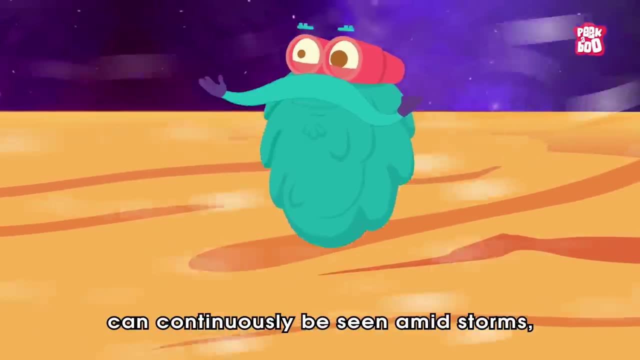 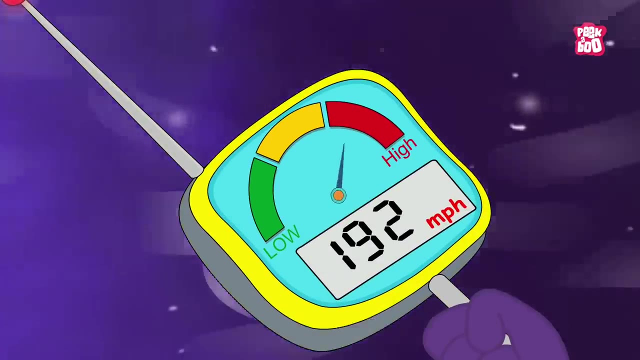 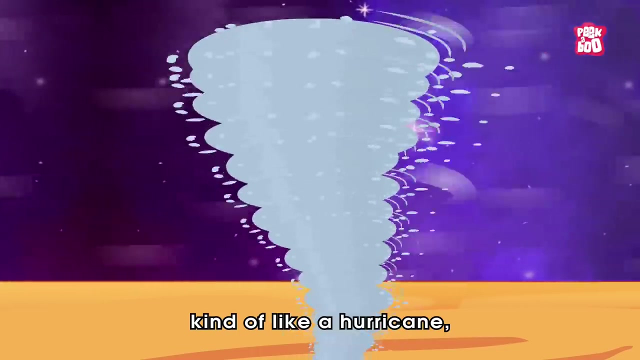 And is surrounded by an ocean of hydrogen and helium gases. Plus the planet's surface can continuously be seen amid storms causing wind with a speed of around 192 miles per hour to more than 400 miles per hour. This storm is massive, kind of like a hurricane. And at its widest point, the storm is about three and a half times the Earth's diameter. On top of that, the atmosphere on Jupiter is very thick, which is composed of a mixture of hydrogen helium and much smaller amounts of methane and ammonia. 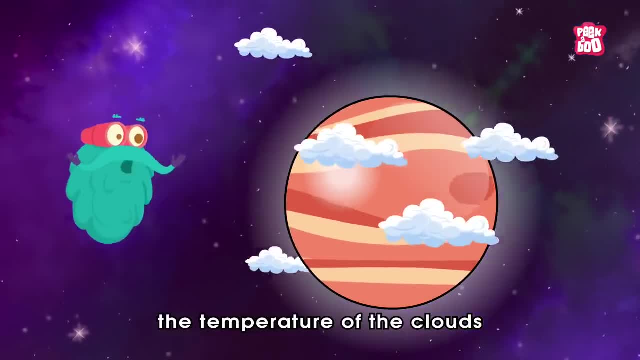 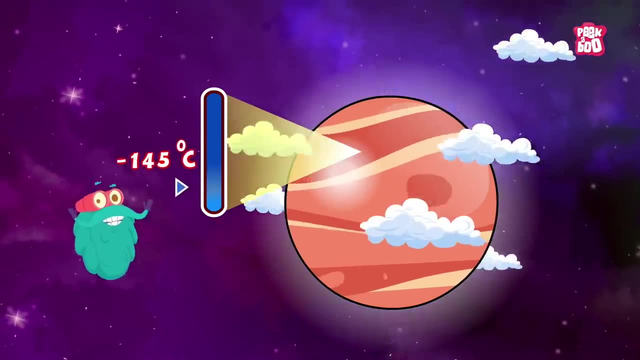 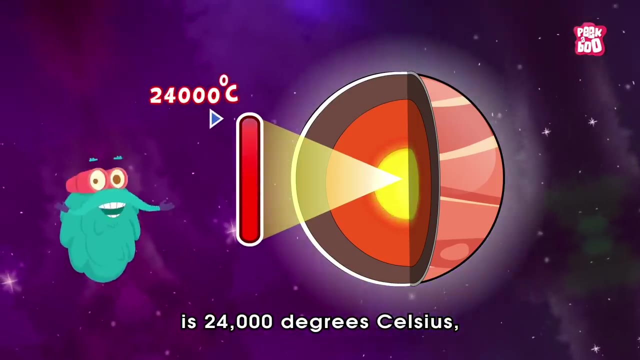 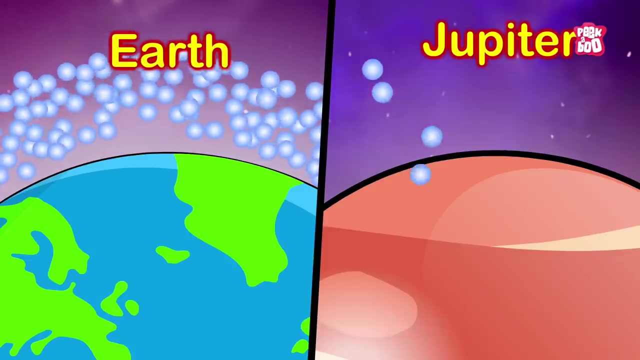 Also, the temperature of the clouds surrounding Jupiter is minus 145 degrees Celsius. On the contrary, the temperature of its inner core is 24,000 degrees Celsius, which is hotter than the Sun itself, Due to its hot core, hydrogen, which is in a gaseous form on the Earth.